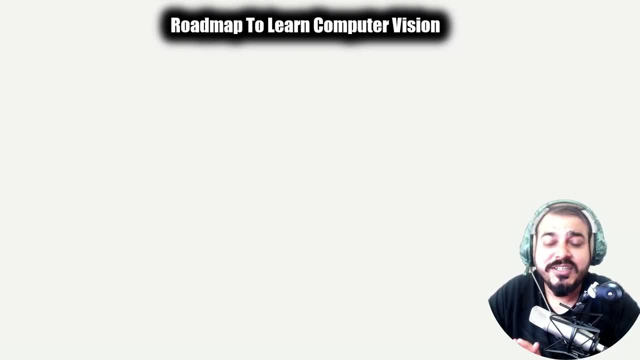 Hello, all my name is Krishnayak and welcome to my YouTube channel. So, guys, today, in this particular video, I'm going to discuss about the roadmap to learn computer vision. Now, whenever I talk about computer vision, guys, at the end of the day, your input data set will be: 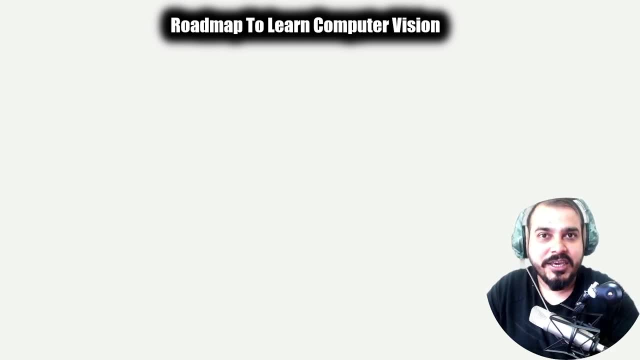 in the form of images and video frames. So any application that you're probably developing when your input data is in the form of images or video frames, any type of image processing that you want to do, any type of deep learning solution that you really want to create, that all will definitely. 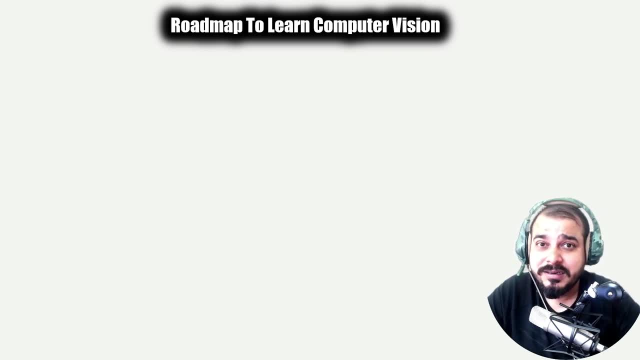 be coming in the part of the computer vision, And computer vision has a huge scope. There are many jobs available related to it and there are many, many companies who are creating some amazing stuff with respect to computer vision. Now, in this video, we'll try to focus on the entire. 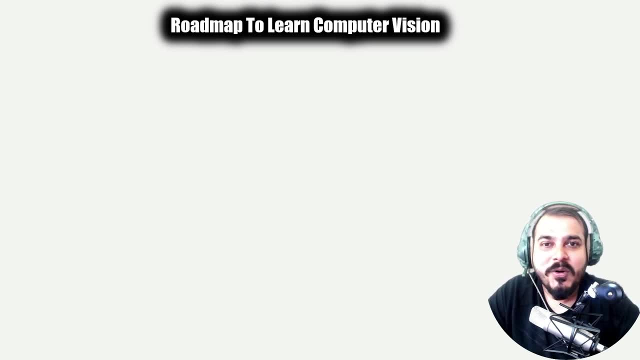 roadmap. And again, guys, I usually first of all upload all the videos in my channel and then only I go with the roadmap. So whatever I'm showing you over here, some or the other way, the videos have been uploaded in my channel, Okay, so let's go ahead without wasting any time. If you're new, 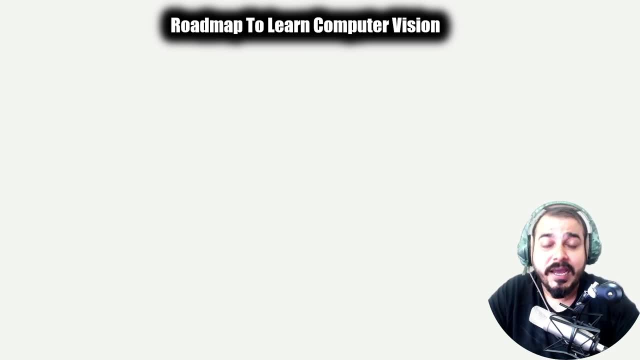 to my channel. please make sure that you subscribe to the channel. press the bell notification icon. So let's start with the basic thing. You know, wherever, whatever you study, guys, first thing is that you really need to cover the basics Now, in basics, with respect to computer vision. 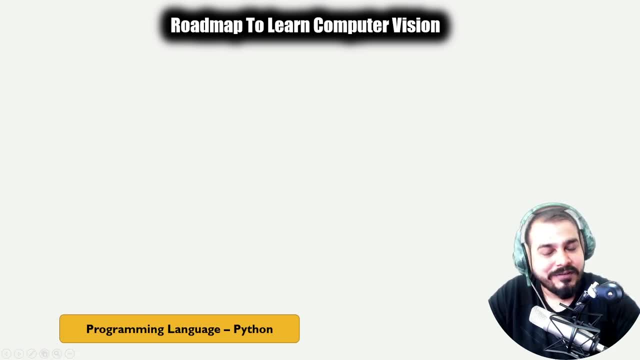 what all things are getting included. One is programming language. Definitely you have to learn about Python, because Python has some amazing libraries. With the help of computer vision also, it has some amazing cool libraries through which you can do a lot of image processing. You can. 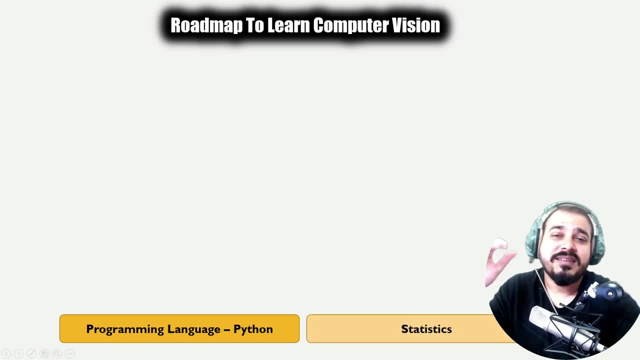 different filters, also Along with Python, again. the other basic thing that you really need to be strong is statistics. Why? Because statistics concepts will get applied in some of the techniques like image processing and some of the analysis with respect to images itself. right, 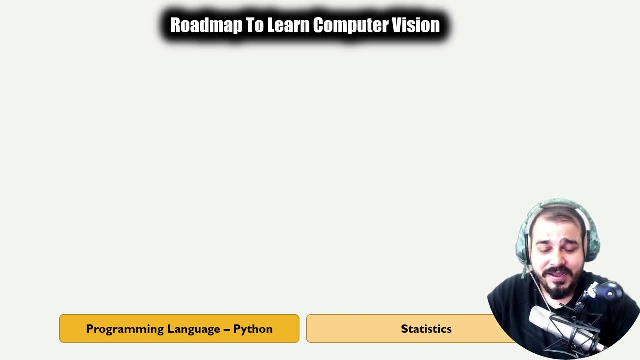 So this too is must basic things right Now. similarly, one more base you really need to cover, okay, And that is nothing but introduction to neural network. See, at the end of the day, whenever I say computer vision, right, Some or the other way, you're going to apply deep. 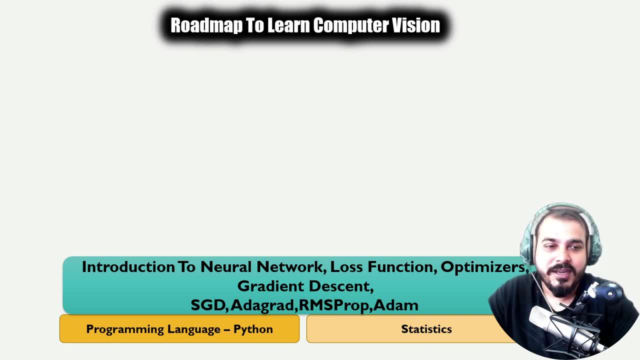 learning techniques like conversation, neural network, object detection and all right. So for that, whatever technique you apply, let's say that tomorrow you want to run RNN also right, These are the basic things. If you learn Hugging Face Transformer, if you learn, probably, any advanced, 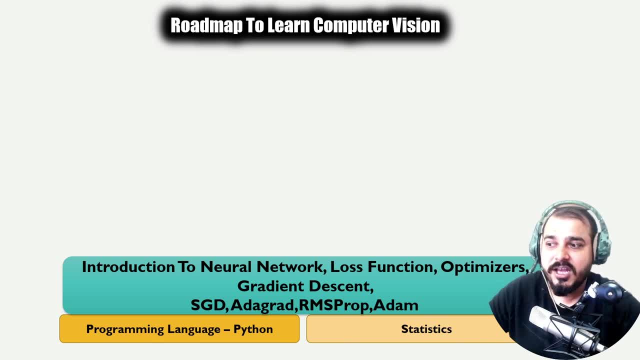 technique also. these are the basic things that you really need to be strong at. You need to know about loss function optimizers like gradient descent, stochastic gradient descent, Adagrad, RMS, prop atom optimizers, different, different kind of activation function- And this is super. 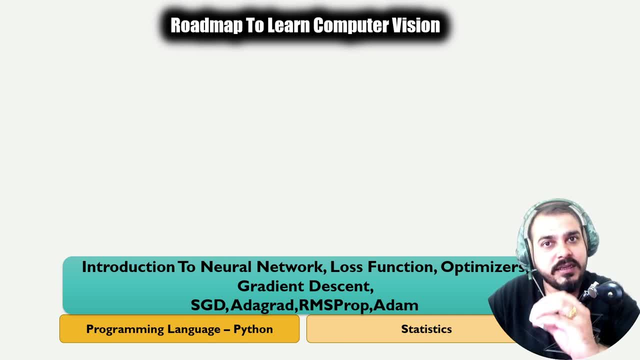 very strong before you go ahead. you know, Because at the end of the day, some or the other thing will be getting used in deep learning techniques, like wherever convolutional neural network will be actually coming right, And at the end of the day, we will be using convolutional neural network. 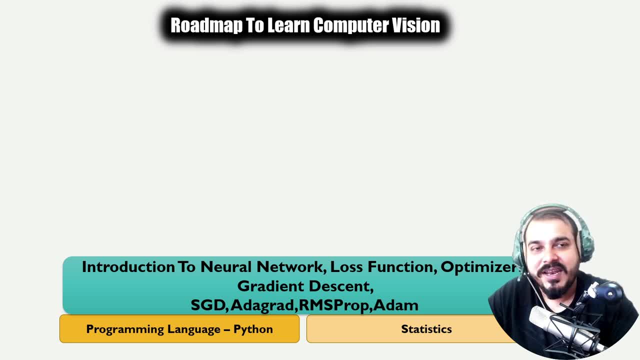 or the advanced techniques like transfer learning or object detection, whenever your input data setting is in the form of images or video frames. okay, Now coming to the next step here. the next thing is that you really need to understand: how does artificial neural network work? Try to solve. 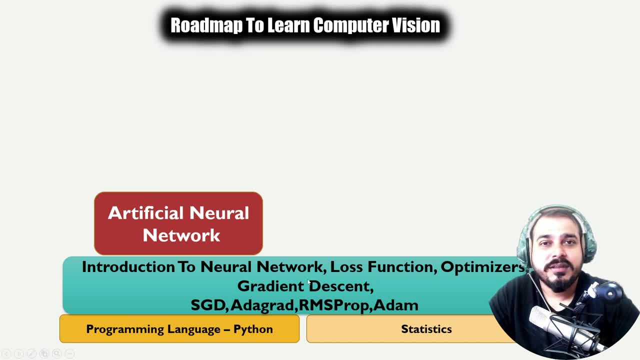 some of the end-to-end applications with the help of your computer. So let's get started. So let's go ahead, Start with proper business skills and take a look at 그. What isалfe Image processing? now, what exactly is image processing? Let's say, guys, I've got an RGB image, I apply different. 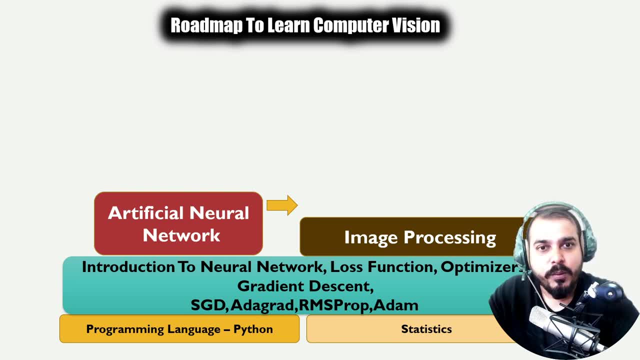 different filters and I know that what kind of output I'll be able to get from that particular filters, You know it can be image masking, it can be object detection, It c an be different, different things, different different kind of filters on the top of images and you'll be getting some kind of 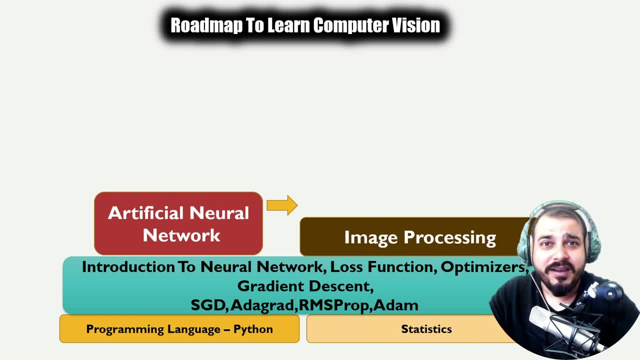 output of that specific image. it can be a shadow, it can be, uh, different, different filters, like they are. filters like to find out the vertical lines, to find out round circle many things as such. right, so this image processing will be able to help you to with the entire image analysis. okay, 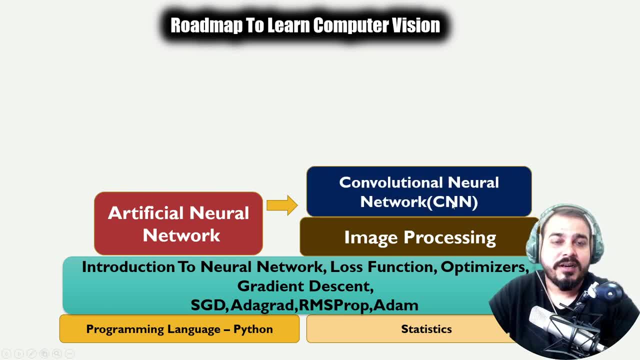 now coming to the next one: convolutional network. now, whenever you really want to solve any problem like image classification, you know, like how many images are there, what, what kind of image this is? you know not how many kind of image, but what image this is like, suppose, if i say there is a image of 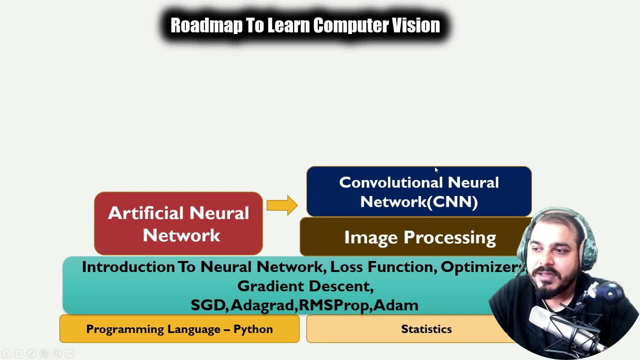 a cat, dog or monkey, it should be able to determine right. for that you definitely require convolution neural network and again, i've created all this particular playlist in my deep learning playlist, which is super, super important at the end of the day. in this also, your input is basically in the 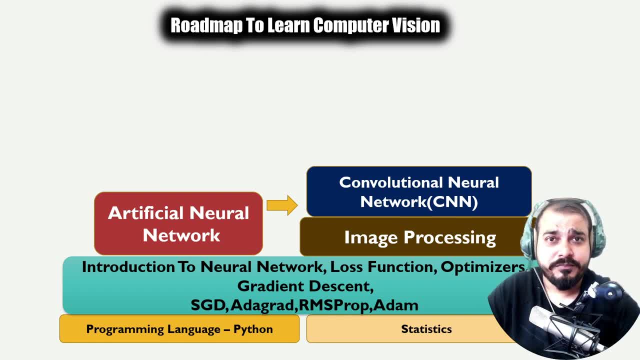 form of images. now let's say that if you have got a video frame right, then how you are basically going to solve this problem is: you are going to have a video frame right and you are going to get the input in the form of images. then again over there, you really need to apply image processing. 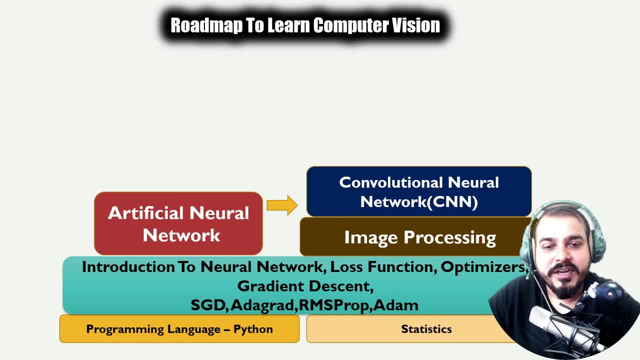 because, with the help of some of the libraries which i'm going to talk about, what it is going to do? it is going to convert that video frames entirely into different, different images, frame by frame. it will just try to do it and how it is done, again by using some image processing. 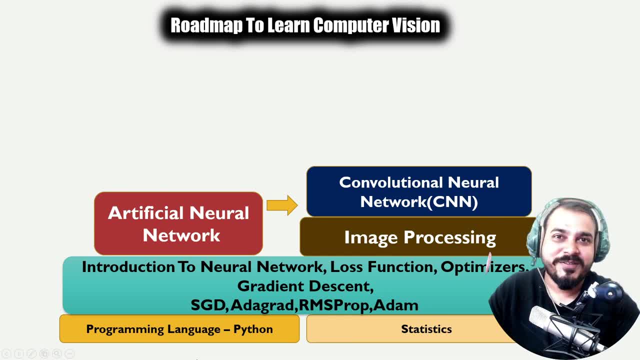 techniques, again with the help of python programming language, again with the help of some of the libraries which i'm again going to talk about it. okay, so coming to the convolutional network, it will definitely help you to deal with the image classification problem statement. then there is a second one, which is the image classification problem statement. 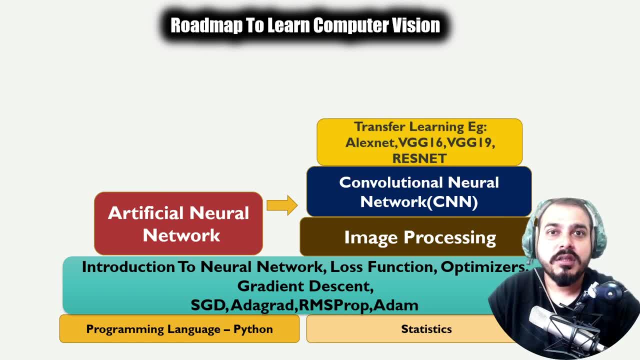 there is also called as transfer learning techniques, and these are some state of art algorithm which actually help you with image classification, because most of the time people ask that which, how many number of hidden layers i should use in convolutional network, how many number of convolution layer i should i use in how many number of max pulling layer or min pulling? 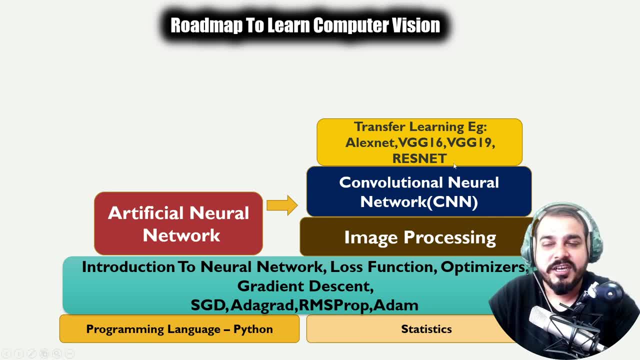 layer. i should basically use it. so for that particular case, we basically use transfer learning technique. these are some of the state of art algorithm and this they have worn. basically the image net classification problem statement. so you can basically use the image classification problem statement. you can use this same transfer learning technique, use the exact same way. 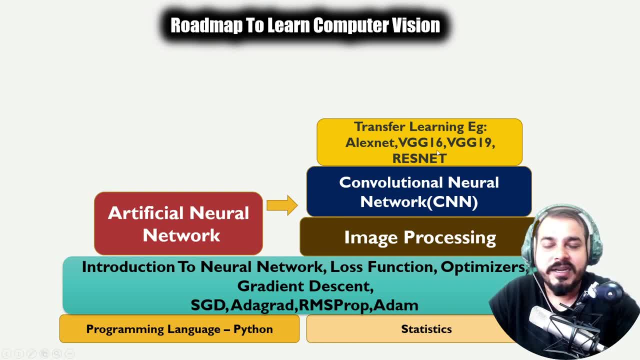 to change the number of outputs and then you can basically train your entire data set from scratch. okay, so transfer learning technique is also super important. now, after you probably cover transfer learning technique, then you go with object detection, like rcn and shd. yolo, right. here you're specifically solving use cases related to object detection, right? 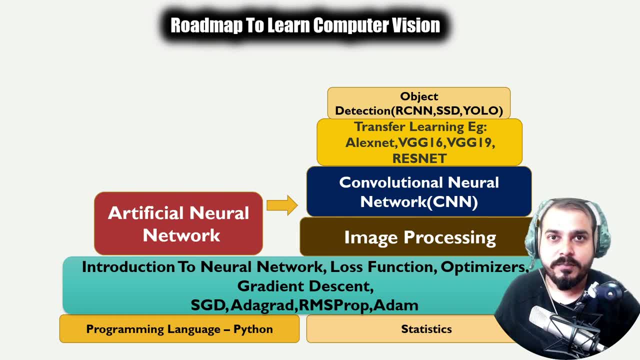 some of the examples may be right. uh suppose, let's say there is a factory, you know number of items that are coming inside the factory. it should be able to detect that particular item and should be able to increase the counter right some of the applications that i have. 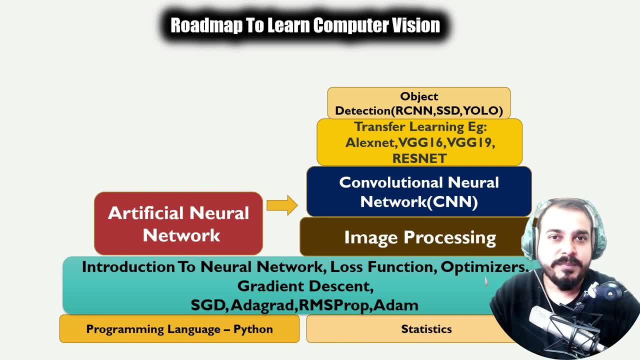 personally done in my previous companies. right, uh. so in the basement that actually put a camera, it should be able to detect whether the person is wearing a helmet or not. whoever is coming in the basement, right, and based on that, that notification can go to that specific person face image.